Professor Dave here, let's graph some circles. 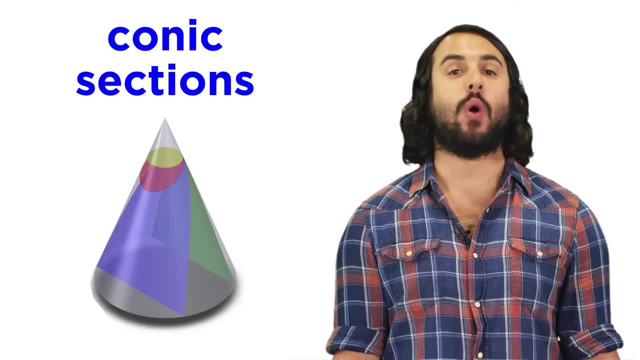 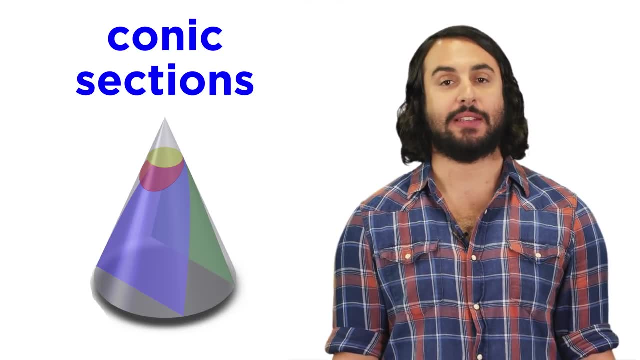 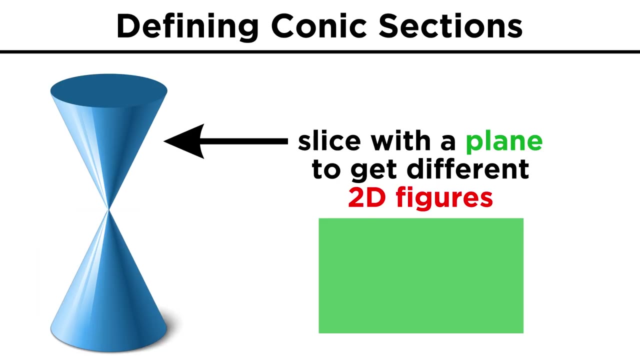 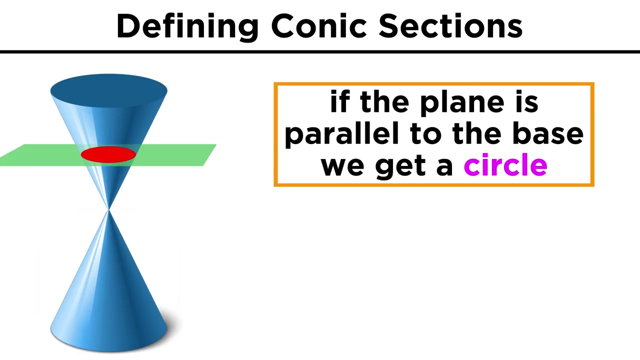 In algebra, there are so many things that we could graph, but there is one class of figures called conic sections that will be very important. First, let's learn what this term means. Take this three-dimensional, right, circular, double-knapped cone. We can create different two-dimensional figures by taking a plane and swiping through the cone in different ways. If the plane goes from one side of the cone to the other, and is parallel to the base, we get a circle. 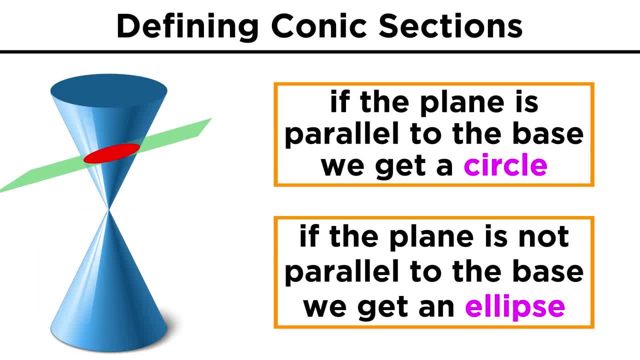 If the plane does the same thing but is not parallel to the base, we get an ellipse. 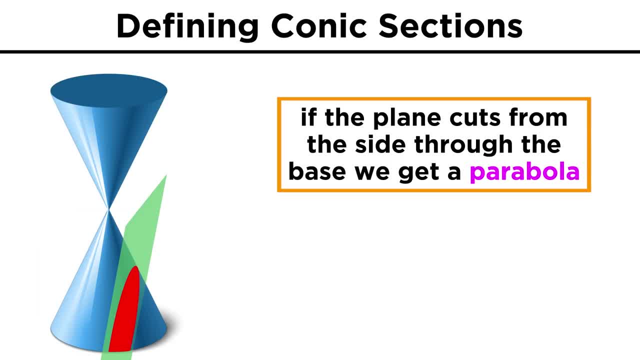 If the plane cuts from the side of the cone down through the base, we get a parabola. 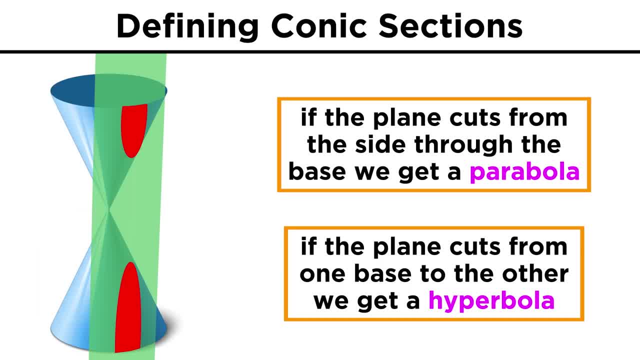 And if the plane cuts all the way from one base to the other, we get a hyperbola. 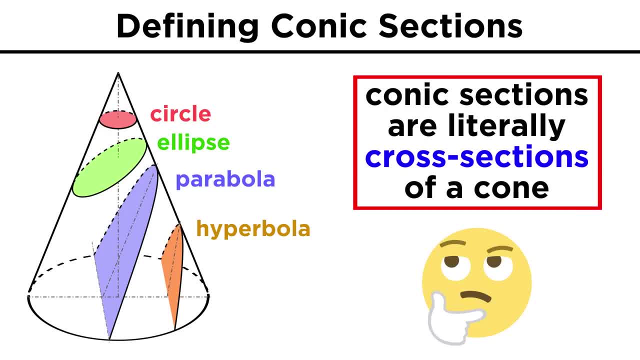 So these are called conic sections because they are literally different cross sections of a cone. 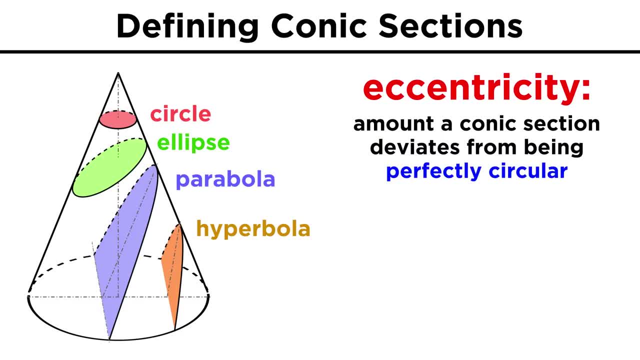 We can also describe these using a parameter called eccentricity, which is a term that describes how much a conic section deviates from being perfectly circular. For a circle, this value is zero. 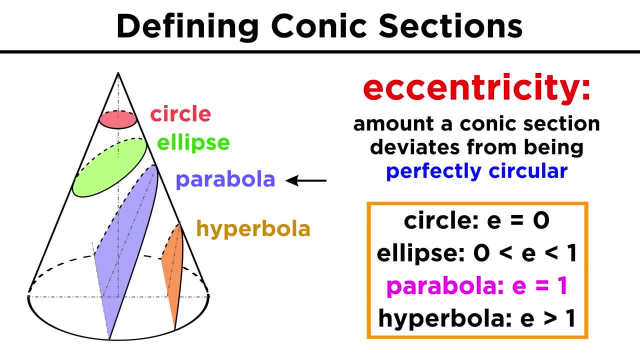 For an ellipse, it's between zero and one. For a parabola, it's precisely one. And for a hyperbola, it's precisely one. 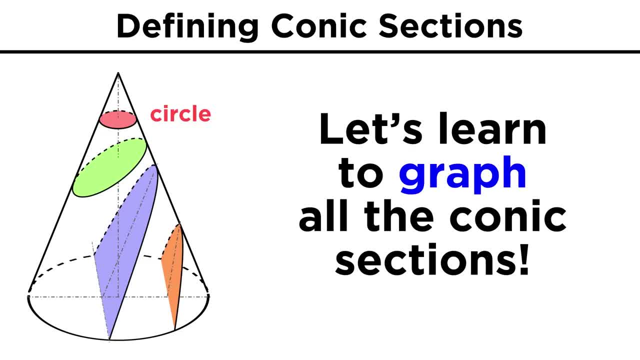 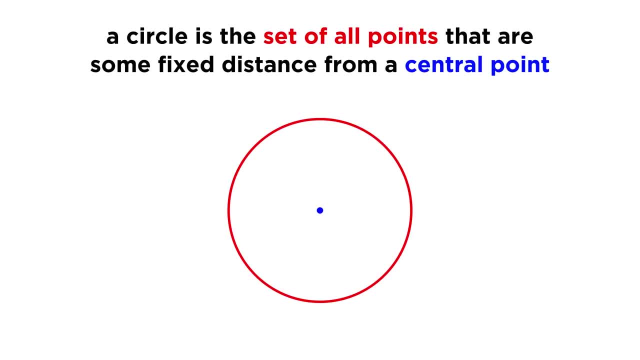 For a hyperbola, it's greater than one. Let's learn how we can graph these different figures, one at a time, starting with circles. As we know, circles are defined as the set of all points in a plane that are equidistant from a fixed point, which we refer to as the center of the circle. This distance from the center to any point in the circle is called the radius of the circle. 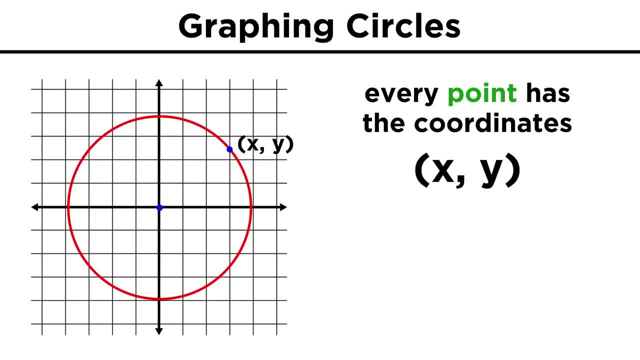 If we place the circle in the coordinate plane, we get the radius of the circle, and if we start from the center, we could say that any point on the circle has coordinates of , because any point on the circle contains x and y values that satisfy the conditions of the circle. 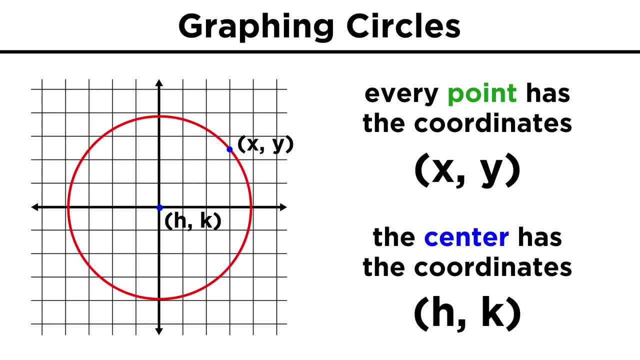 We can also label the center as the point . So how can we algebraically represent the set of points in the circle? 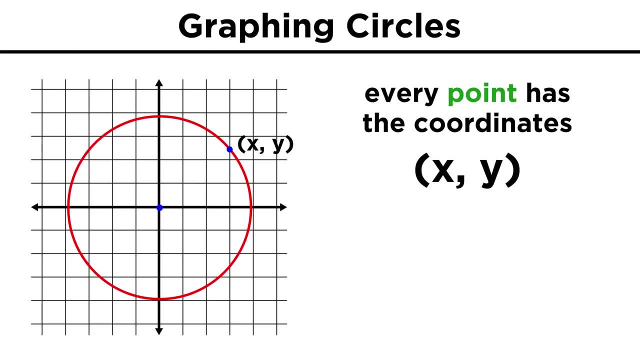 circle. If we place the circle in the coordinate plane, we get the radius of the circle, and if we place the circle in the coordinate plane, we get the radius of the circle. We could say that any point on the circle has coordinates of, because any point on 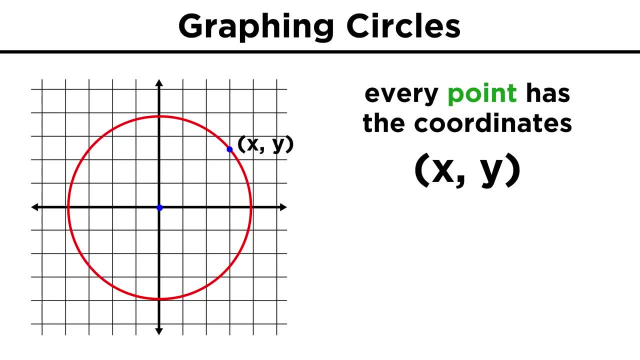 the circle contains X and Y values that satisfy the conditions of the circle. We can also label the center as the point. So how can we algebraically represent the set of points in the circle? Well, we just learned how to use the distance formula. again, that looks like this, and it: 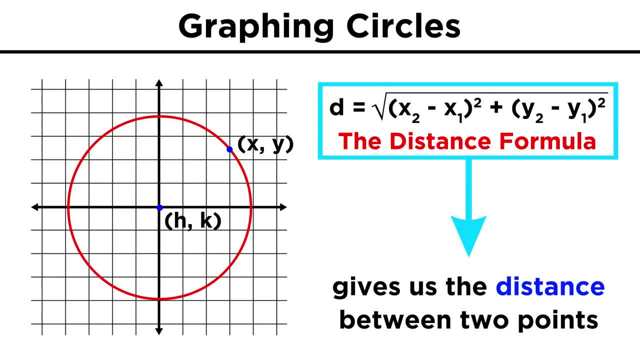 says that when we examine any two points, they are equal, So we can just use the distance formula. Again, that looks like this: And it says that when we examine any two points, they are equal, We can just use the distance formula. Again, that looks like this: And it says that when we examine any two points, they are equal, So we can just use the distance formula. And it says that when we examine any two points, they are equal, We can just use the distance formula. 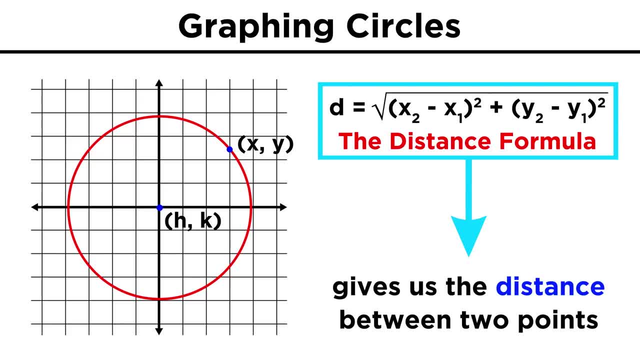 The distance between them will be the square root of the square of the difference between the X values plus the square of the difference between the Y values. This applies here because any point on the circle has coordinates and the center, which is what we are measuring the distance from, will always be HK, so we get the square. 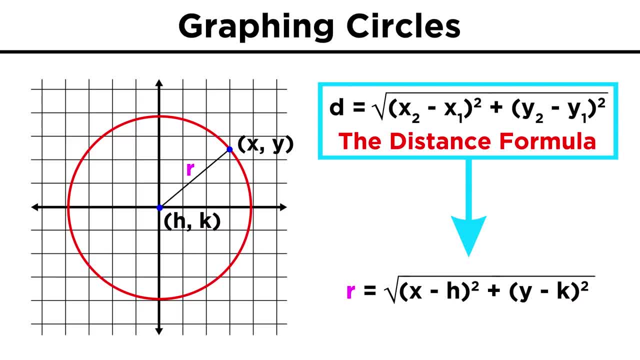 root of quantity squared: плюс plus y, minus k, quantity squared For any x and y values that satisfy this expression. we get some radius of the circle represented by R. All we have to do is square both sides and we get the standard form for the equation. 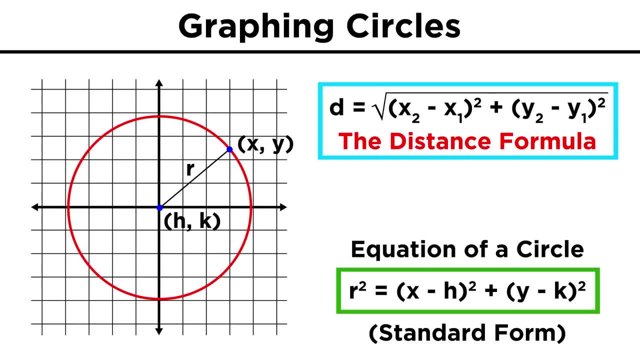 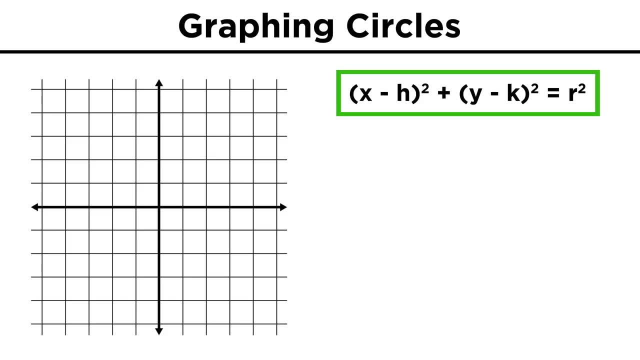 of a circle with three terms all squared. We can use this understanding to graph a circle given an equation. Let's start with something simple like x squared plus y squared equals nine. In this case there are no h and k terms, so h and k must both be zero, meaning that 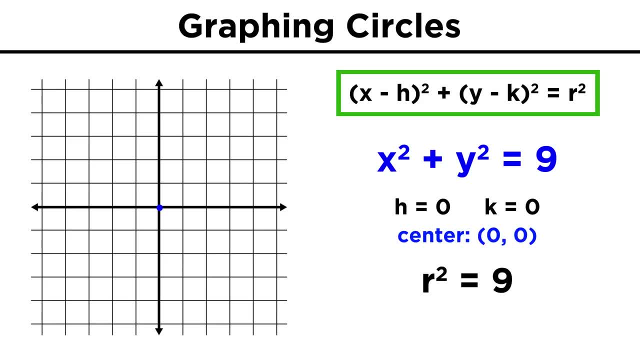 the center of the circle is at the origin. Then R squared is nine, so the radius must be three, and there's our circle. Now let's look at one with h and k terms present Here. the only thing we have to remember is that it's x minus h and y minus k. 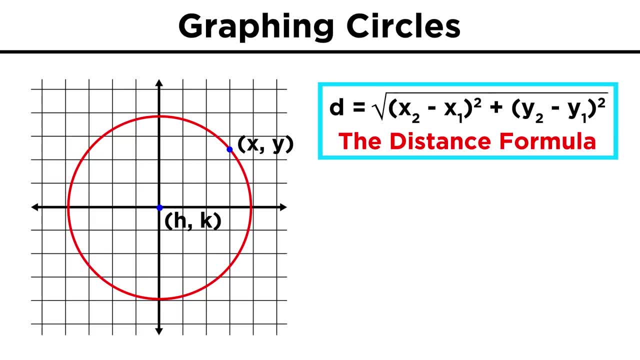 Well, we just learned how to use the distance formula. Again, that looks like this, and it says that when we examine any two points, they're not equal. 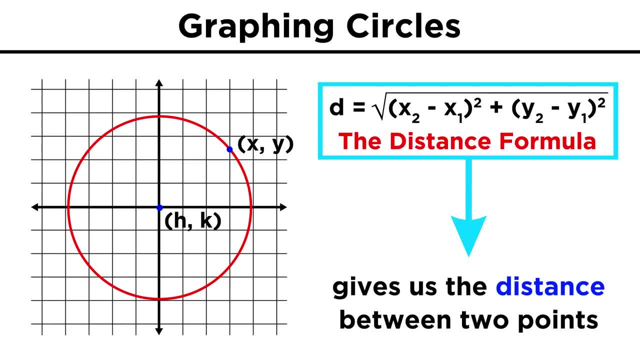 in the coordinate plane, the distance between them will be the square root of the square of the difference between the X values plus the square of the difference between the Y values. 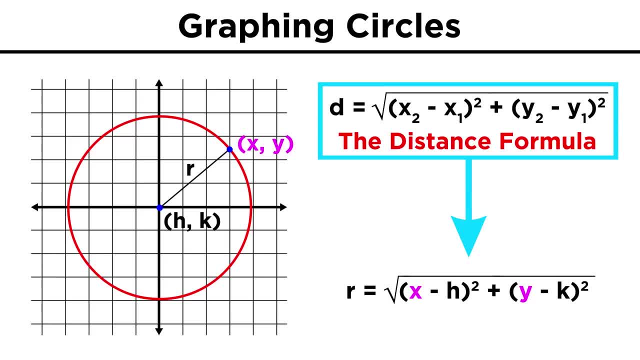 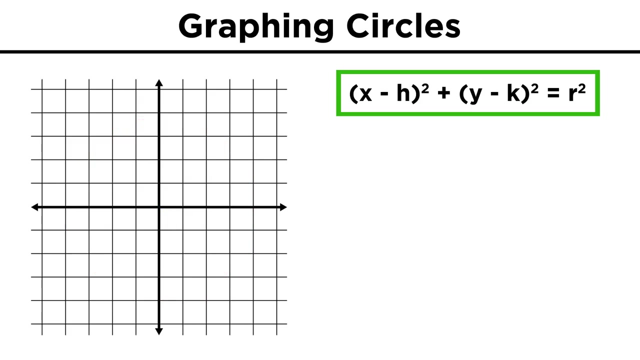 This applies here, because any point on the circle has coordinates and the center, which is what we are measuring the distance from, will always be HK, so we get the square root of quantity squared plus quantity squared. For any X and Y values that satisfy this expression, we get some radius of the circle, represented by R. All we have to do is square both sides, and we get the standard form for the equation of a circle, with three terms, all squared. 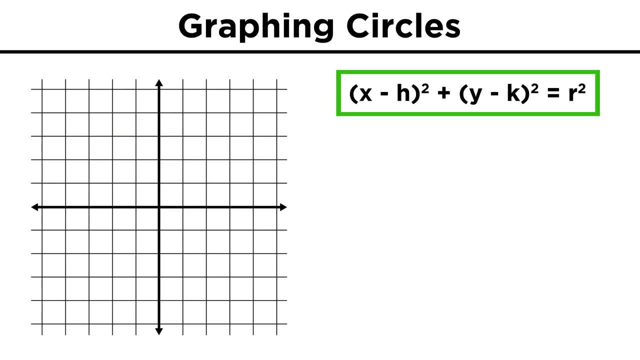 We can use this understanding to graph a circle given an equation. Let's start with something simple, like X squared plus Y squared equals nine. In this case, there are no H and K terms, so H and K must both be zero, meaning that the center of the circle is at the origin. Then R squared is nine, so the radius must be three, and there's our circle. 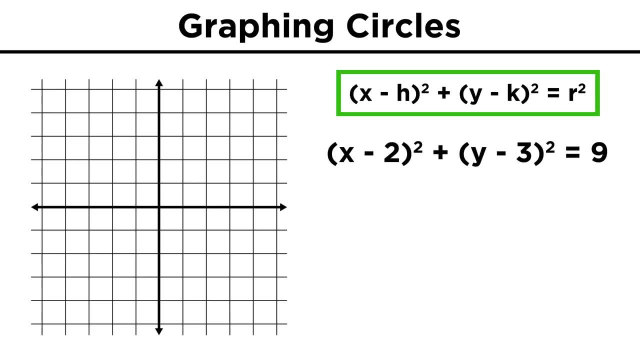 Now let's look at one with H and K terms present. Here, the only thing we have to remember is that it's infinite. It's infinite. It's infinite. 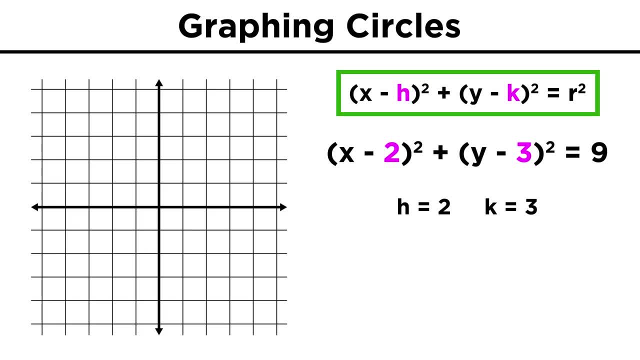 X minus H and Y minus K. So if we have X minus two and Y minus three, the center will be at , both positive, because H equals two and K equals three, according to the equation. 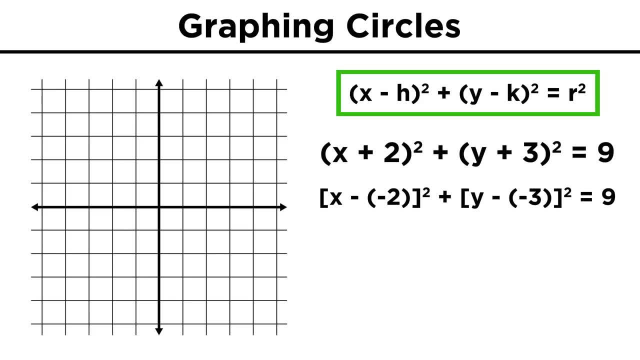 If we had X plus two and Y plus three, that would be the same as X minus negative two and Y minus negative three, so in that case, the center would be at negative two and negative three. 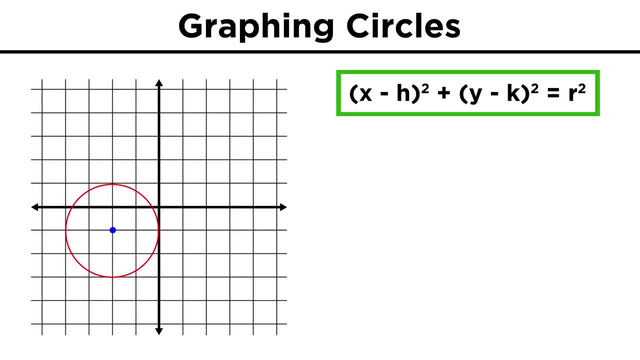 We can also go the other way around and derive the equation of a circle from its graph. Look at this one here. All we need to do is locate the center to get the H and K values, and then find the radius. 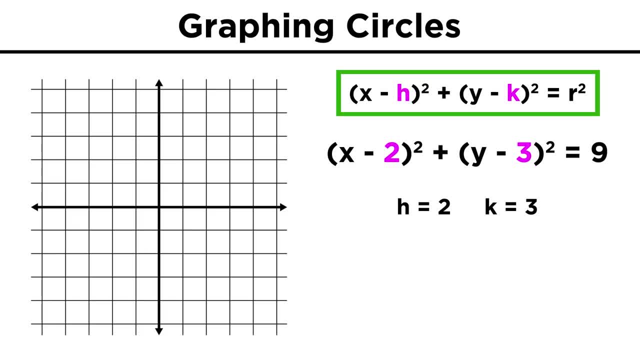 So if we have x minus two and y minus three, the center will be at two- three, both positive, because h equals two and k equals three. according to the equation, If we had x plus two and y plus three, that would be the same as x minus negative two. 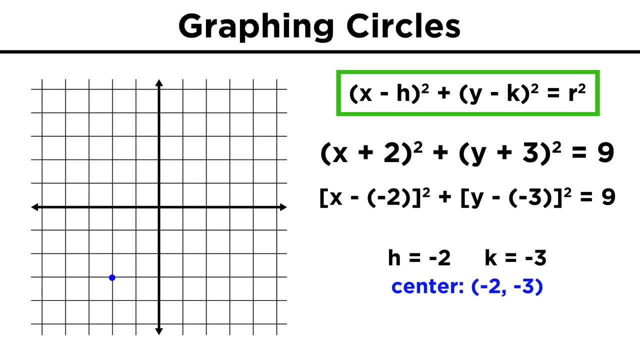 and y minus negative three. so in that case the center would be at negative two, negative three. We can also go the other way around and derive the equation of a circle from its graph. Look at this one. here All we need to do is locate the center to get the h and k values and then find the. 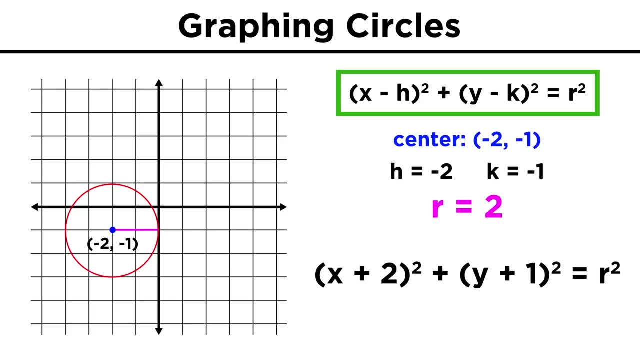 radius. This is easy if we just go in a direct horizontal or vertical direction from the center and see how far it is to a point on the circle. Don't forget to square this, since we need R squared, So this will be the equation. 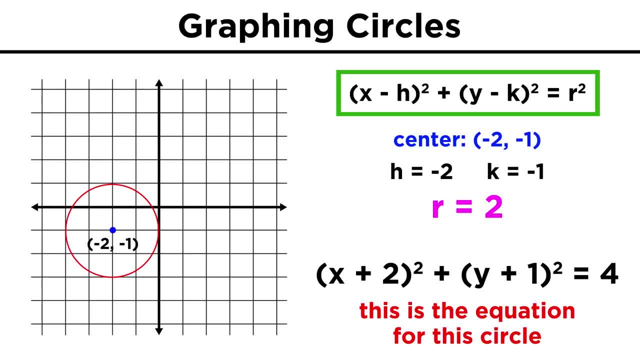 A lot of circles will have graphs and equations that are this simple, but sometimes we have to get clever. Say, we have something like x squared plus y squared plus four, x minus six, y minus twenty-three. If we look carefully, we will notice that this can be rearranged to put into standard. 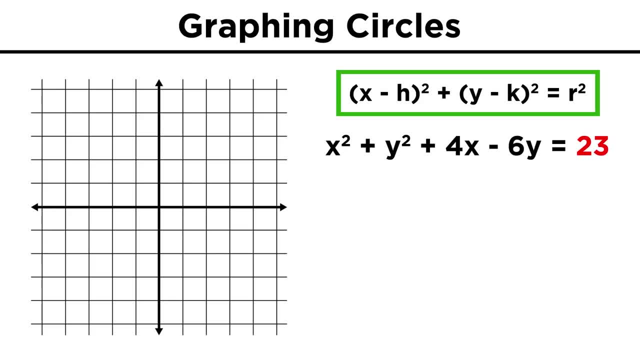 form. We can just bring twenty-three to the other side and then group the x and y terms separately. Earlier in this course we learned how to complete the square, and that's exactly what we will do here, but twice, once per variable. 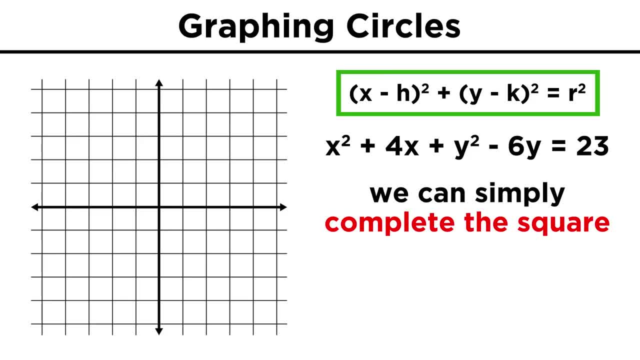 If you need a refresher, go back and check out that tutorial now. Otherwise, we simply notice that for the x terms, we can add four to get a perfect square, making sure to add four to the other side as well, and now this term can become x plus. 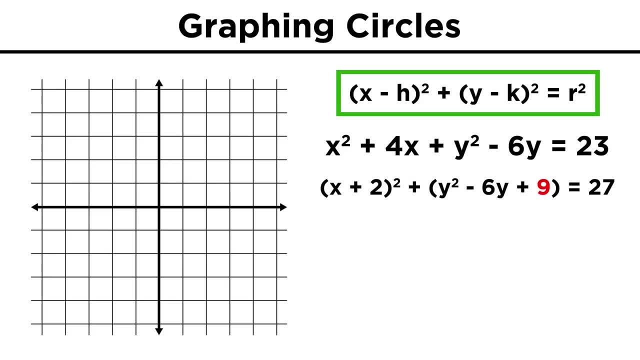 two quantity squared. We can also see that for the y terms we have to add nine again, making sure to add to the other side as well, and again we have a perfect square which allows us to express this as y minus three quantity squared. 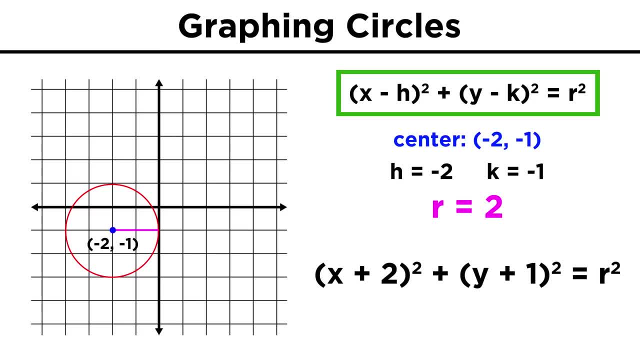 This is easy if we just go in a direct horizontal or vertical direction, from the center, and see how far it is to a point on the circle. 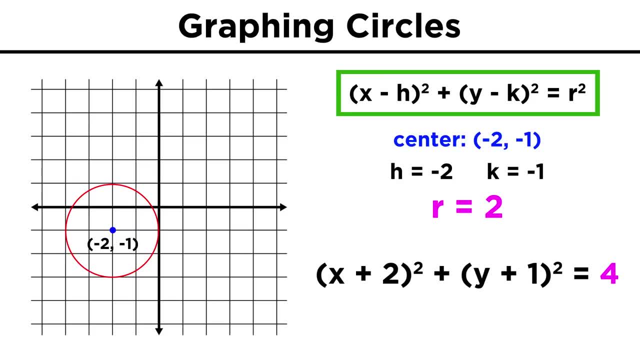 Don't forget to square this, since we need R squared. 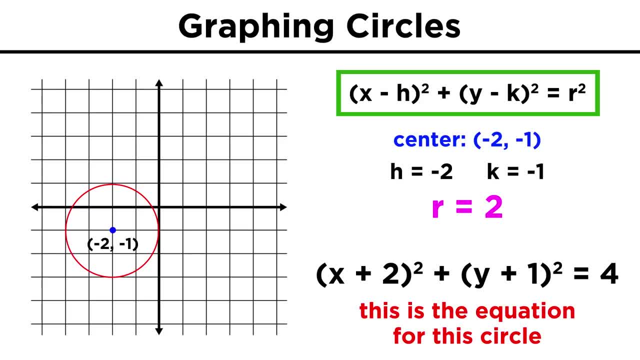 So this will be the equation for the circle. A lot of circles will have graphs and equations that are this simple, but sometimes we have 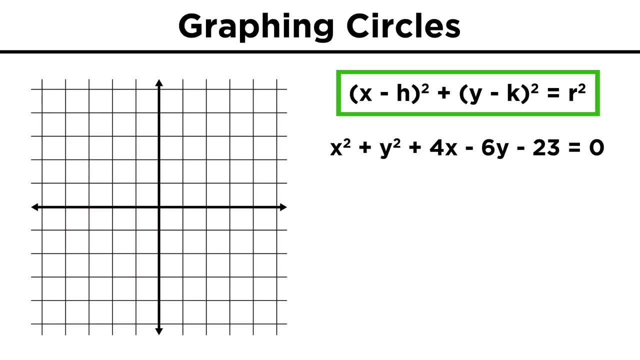 to get clever. Say we have something like X squared plus Y squared plus four X minus six Y minus twenty-three. 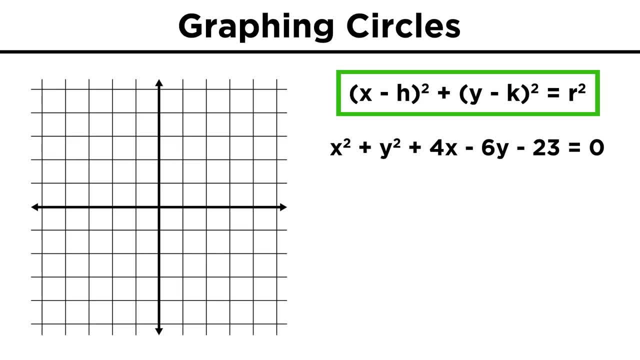 If we look carefully, we will notice that this can be rearranged to put into standard form. 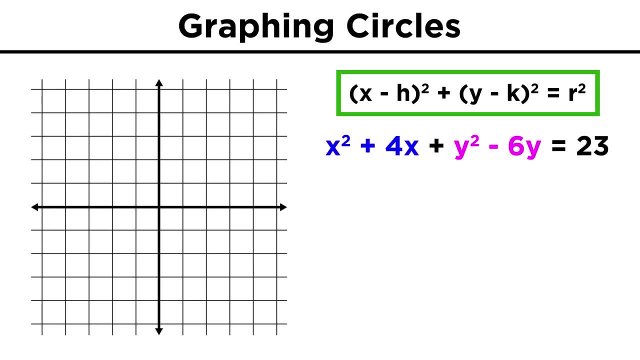 We can just bring twenty-three to the other side, and then group them. 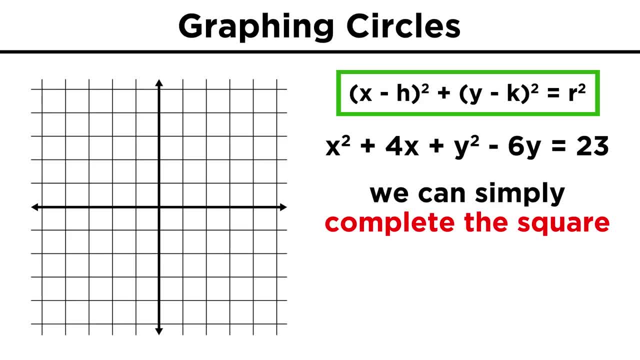 The X and Y terms separately. Earlier in this course, we learned how to complete the square, and that's exactly what we will do here, but twice, once per variable. If you need a refresher, go back and check out that tutorial now, otherwise we simply notice that for the X terms, we can add four to get a perfect square, making sure to add four to the other side as well. And now this term can become X squared. 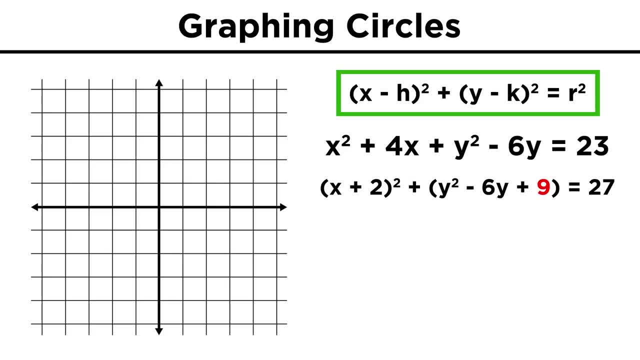 We can also see that for the Y terms, we have to add nine, again making sure to add to the other side as well, and again we have a perfect square, which allows us to express this as Y minus three quantity squared. 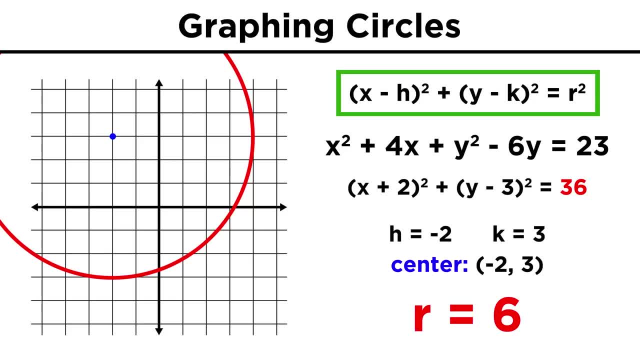 Add up the numbers on the right, and we've got a circle in standard form, with its center 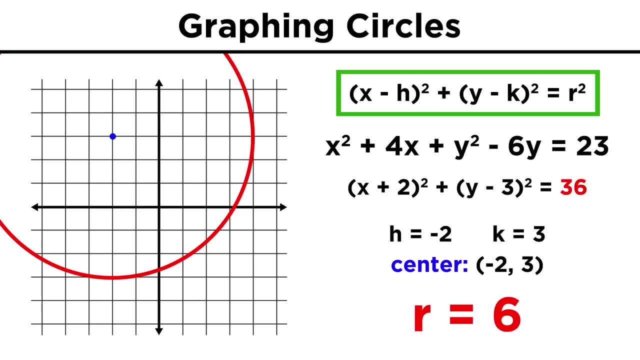 at negative two, three, and with a radius of six. And now let's look at the equation for the Y terms. We can also see that for the Y terms we have to add nine, again making sure to add to the other side as well. 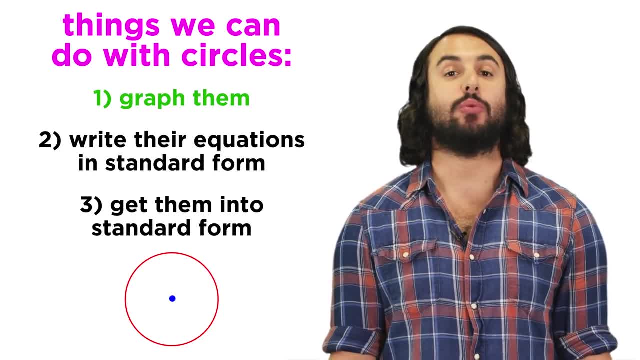 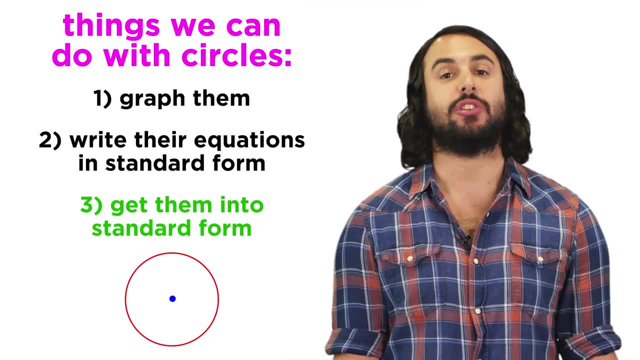 So now we know how to represent circles graphically, how to write their equations in standard form, and how to manipulate an equation in order to get it into standard form, so that we can graph it. 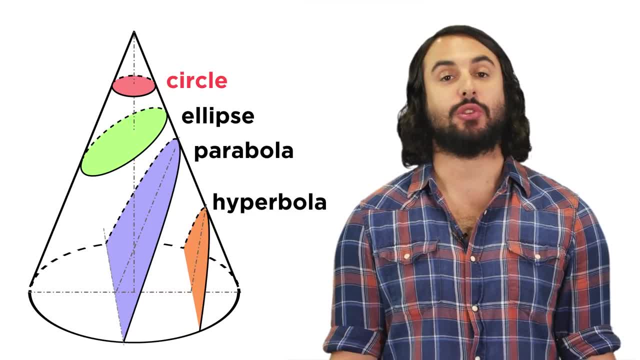 Circles are relatively simple compared to the other conic sections, so let's move forward and check out a trickier one, the ellipse. But first, let's check comprehension.